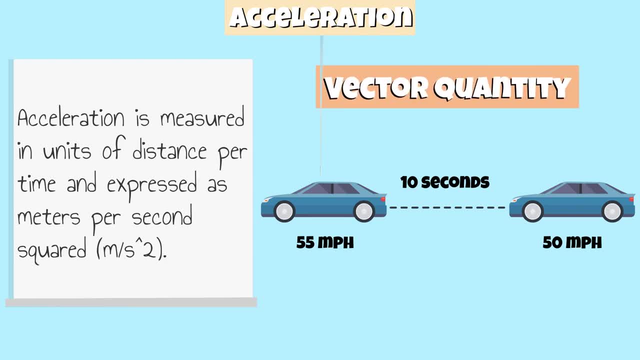 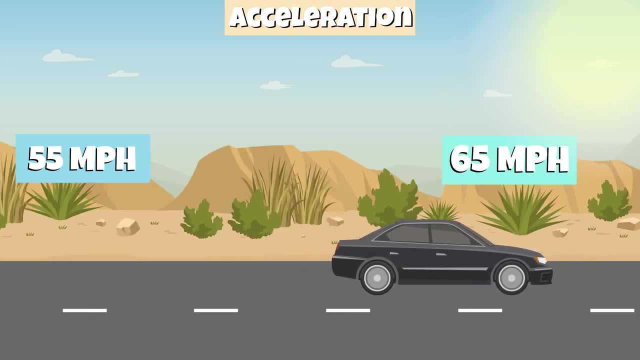 Like velocity, acceleration is a vector quantity. For example, if a car moves slower or faster than the last point of time, then there's a change in acceleration. Now let's talk about the relationship between these three. Speed and velocity are related, but they're not. 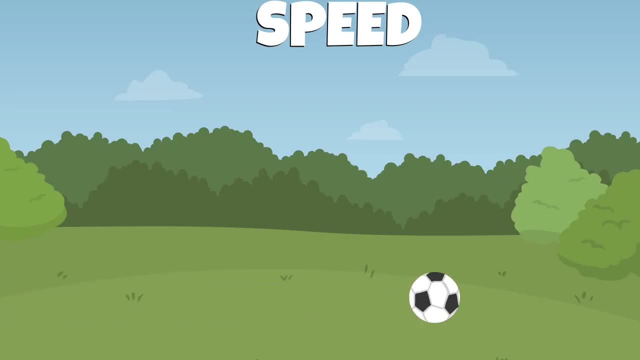 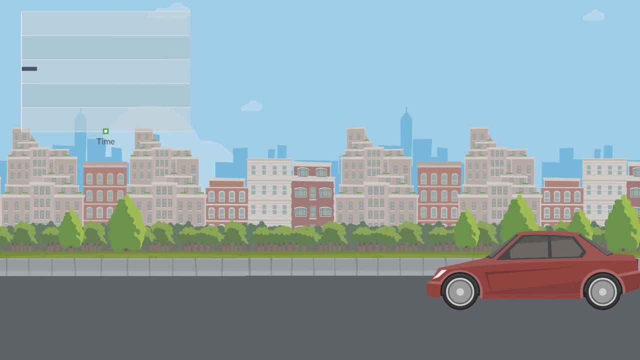 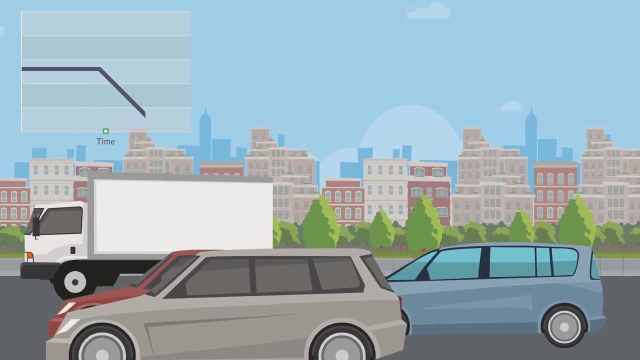 the same. An object can have a constant speed, but its velocity can change if its direction of motion changes. For example, a car traveling at a constant speed of 60 miles per hour in a straight line has a constant velocity, but if the car turns or changes lanes, its velocity. 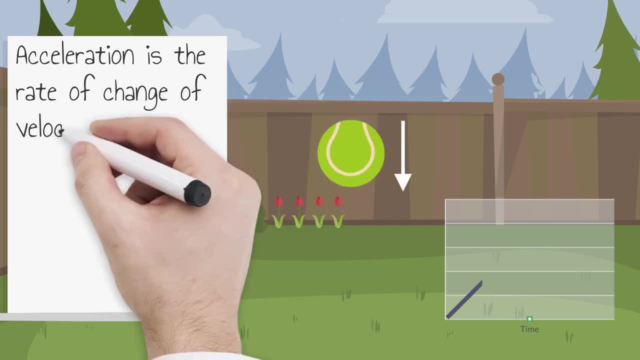 will change. Acceleration is a rate of change of velocity, so an object that is accelerating is changing its velocity. Acceleration is a rate of change of velocity, so an object can have a constant speed but its velocity can change its velocity. 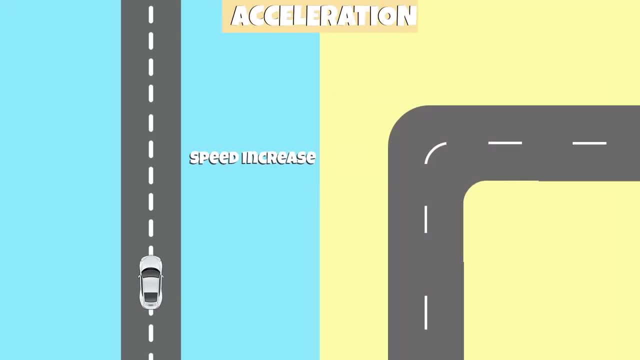 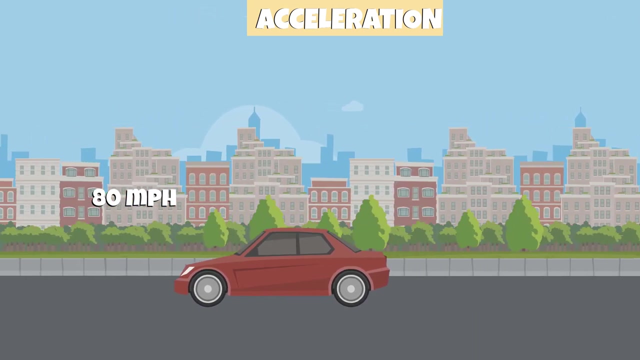 This can happen in two ways. An object can change its speed and since acceleration depends on velocity and velocity depends on direction, a change in direction affects acceleration. For example, a car that speeds up from 60 miles per hour to 80 miles per hour causes 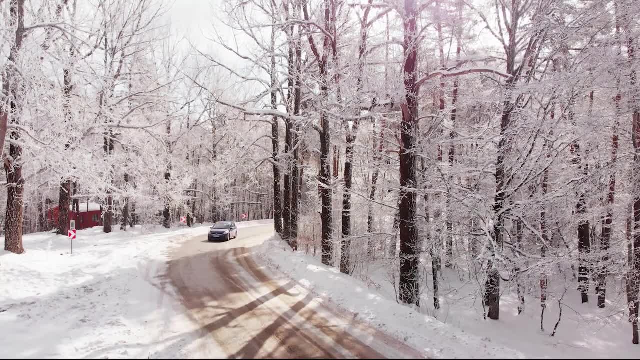 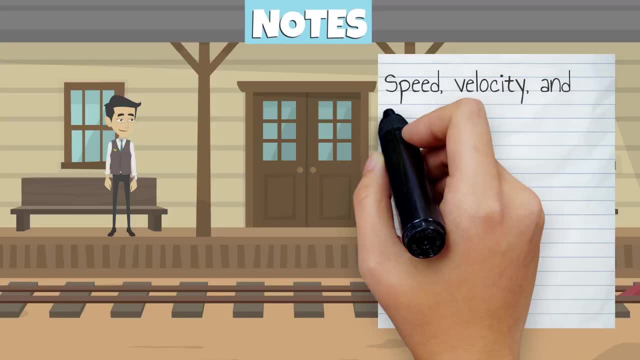 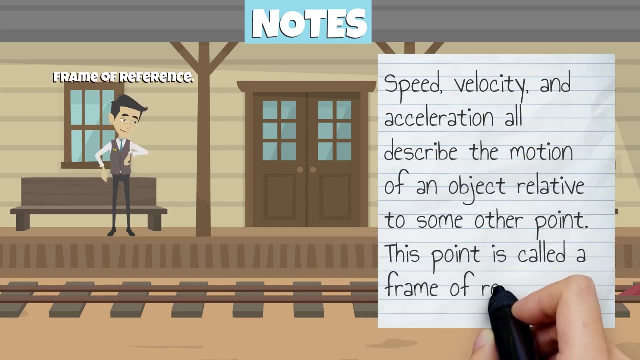 a change in acceleration, as does a car that turns a corner at a constant speed of 60 miles per hour. Let's review what we just learned. Speed, velocity and acceleration all describe the motion of an object relative to some other point. This point is called a frame of reference. Speed is a scalar quantity and measures how 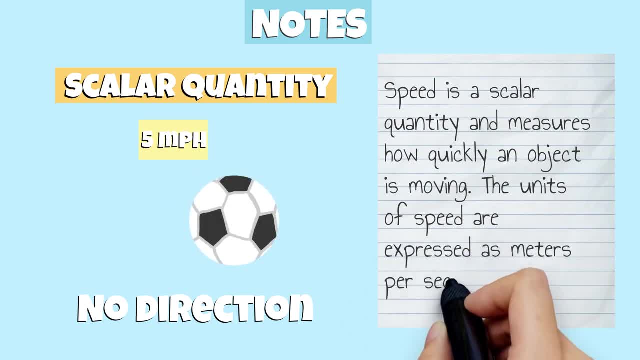 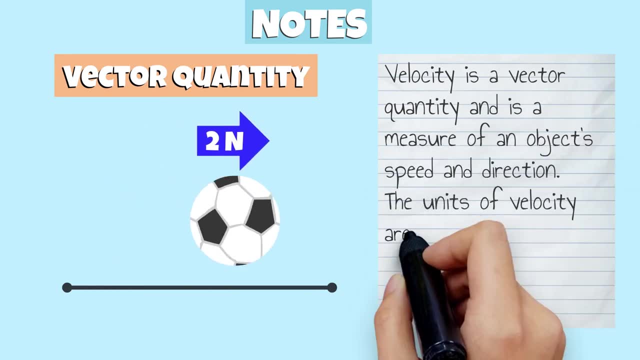 quickly an object is moving. The units of speed are expressed as meters per second. Velocity is a vector quantity and is a measure of an object's speed and direction. The units of velocity are expressed as meters per second. Acceleration is a rate of change of velocity. 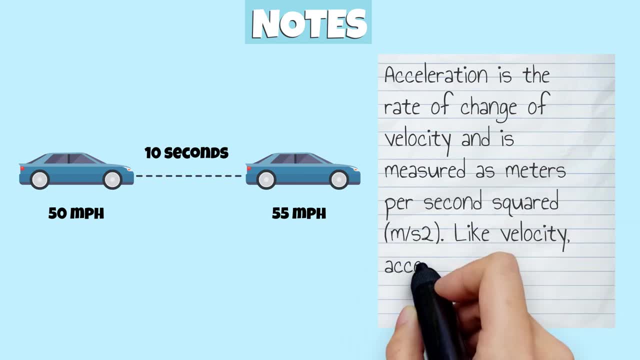 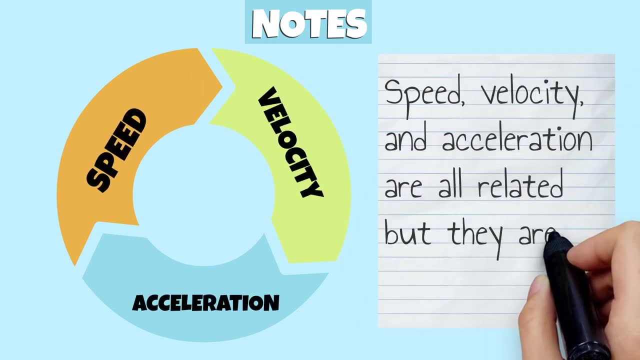 and is measured as meters per second. Acceleration is a rate of change of velocity and is measured as meters per second. per second squared Like velocity, acceleration is a vector quantity. Speed, velocity and acceleration are all related, but they're not the same. An object can have a constant. 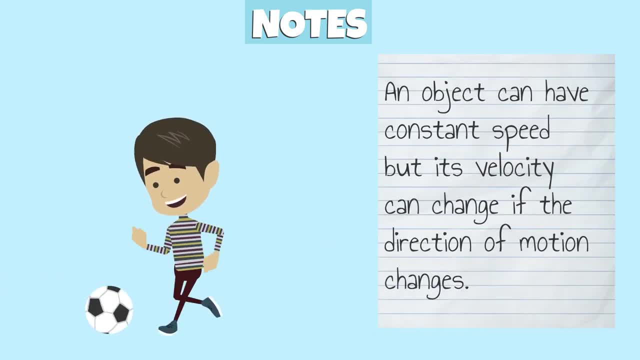 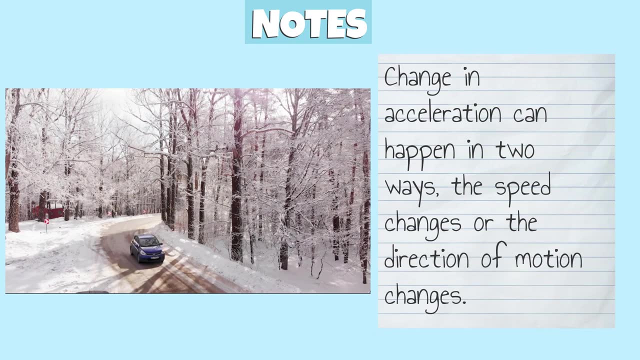 speed, but its velocity can change if the direction of motion changes. Change in acceleration can happen in two ways: the speed changes or the direction of motion changes.